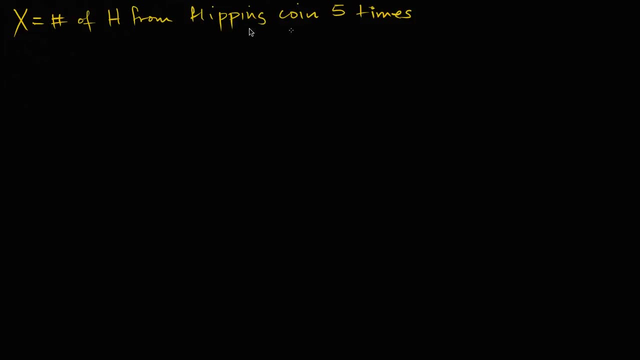 And so, like all random variables, this is taking particular outcomes and converting them into numbers, And this random variable it could take on the value x equals zero, one, two, three, four or five, And what I wanna do is figure out. 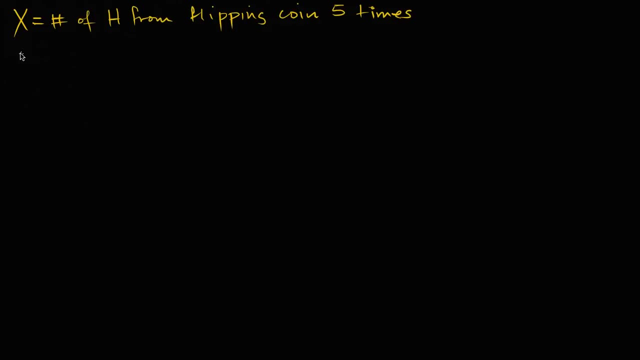 well, what's the probability that this random variable takes on? zero can be one, can be two, can be three, can be four, can be five, And so to do that first, let's think about how many possible outcomes are there from flipping a fair coin five times. 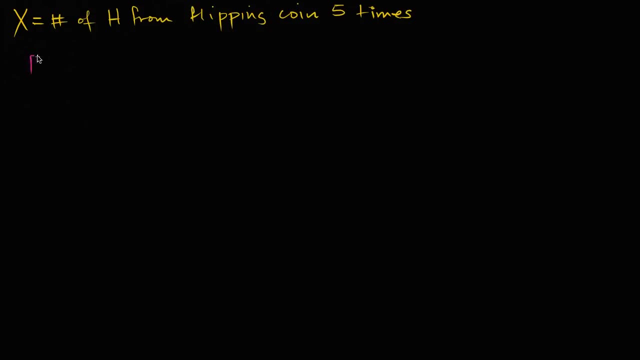 So let's think about this. So let's write possible outcomes, possible outcomes from five flips. From five flips. These aren't the possible outcomes for the random variable. this is literally the number of possible outcomes. for flipping a coin five times, For example, one possible outcome could be: 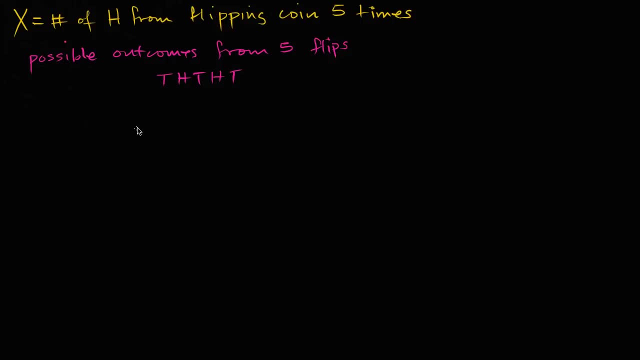 tails, heads, tails, heads, tails. Another possible outcome could be heads, heads, heads, tails, tails, These. that is one of the equally likely outcomes. That's another one of the equally likely outcomes. How many of these are there? 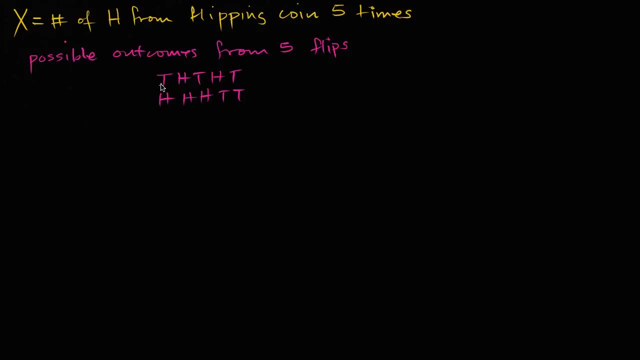 Well, for each flip, you have two. equally, you have two possibilities. So let's write this down. So let me let me so the first flip, the first flip. there's two possibilities: times two for the second flip, times two for the third flip. 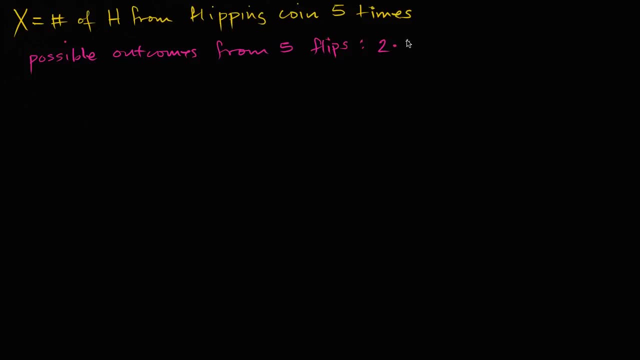 Actually not. let me use a time notation. we might get confused with the random variable Two: two possibilities for the first flip, two possibilities for the second flip, two possibilities for the third flip, two possibilities for the fourth flip and then 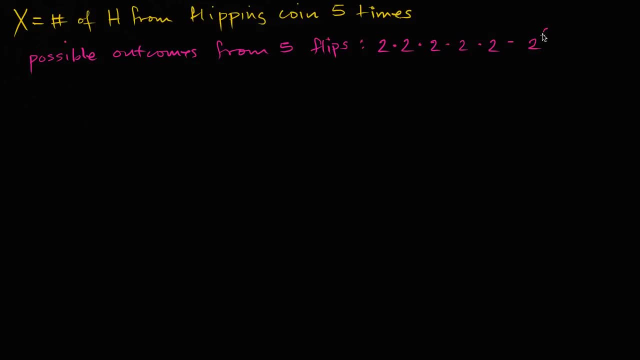 two possibilities for the fifth flip, Or two to the fifth, equally likely possibilities from flipping a coin five times, which of course is equal to 32.. And so this is going to be helpful because, for each of the values that the random variable can take on, 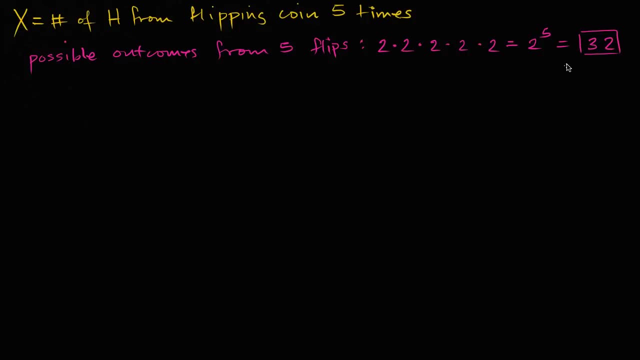 we just have to think about, well, how many of these equally likely possibilities would result in the random variable taking on that value. And let's just delve into it to see what we're actually talking about. All right, and I'll do it in this light. 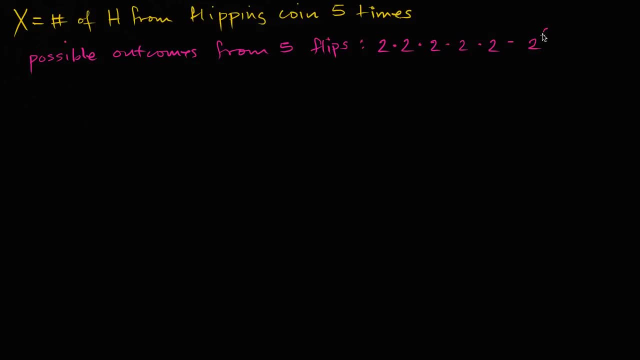 two possibilities for the fifth flip, Or two to the fifth, equally likely possibilities from flipping a coin five times, which is, of course, is equal to 32.. And so this is going to be helpful because, for each of the values that the random variable can take on, 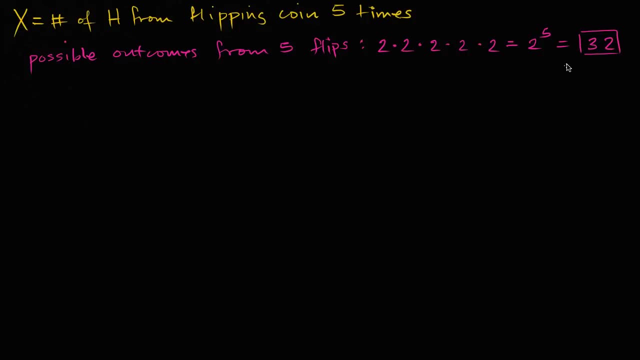 we just have to think about, well, how many of these equally likely possibilities would result in the random variable taking on that value. And let's just delve into it to see what we're actually talking about. All right, and I'll do it in this light. 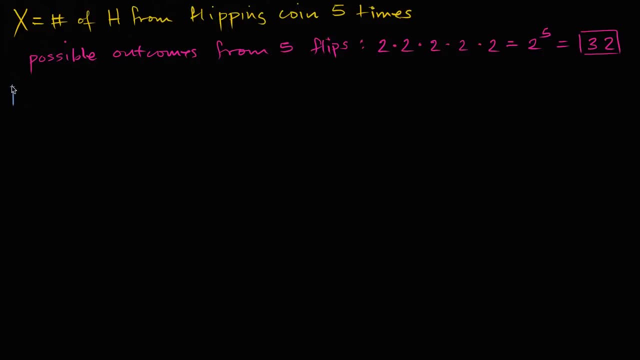 Let me do it in. I'll start it off. I'll start in blue, all right. So let's think about the probability that our random variable x is equal to one. Well, actually, let me start with zero. The probability that our random variable x. 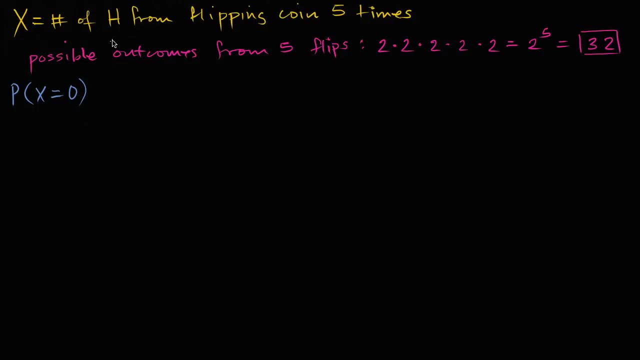 is equal to zero. So that would mean that you got no heads out of the five flips. Well, there's only one way- one out of the 32 equally likely possibilities- that you get no heads, That's the one where you just get five. 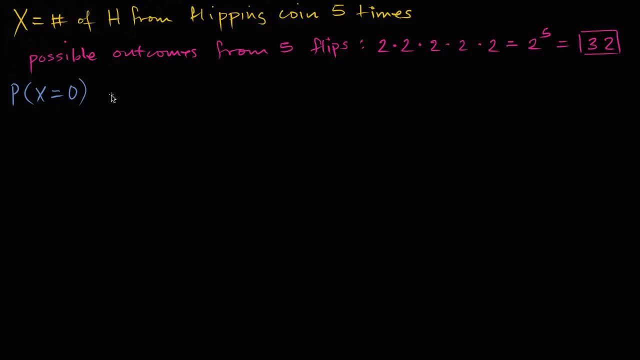 where you get five tails. So this is just going to be, this is going to be equal to one out of the 32 equally likely possibilities. Now for this case, you know to kind of think in terms of kind of the binomial coefficients. 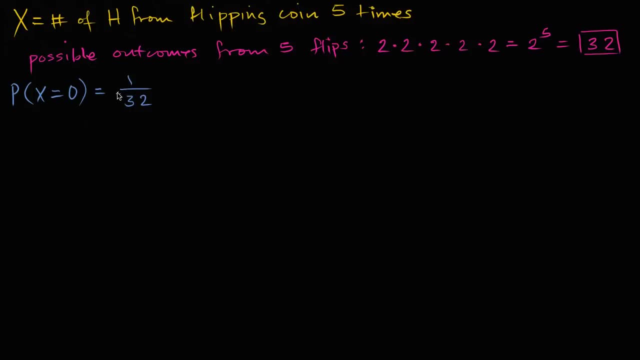 and combinatorics and all of that. it's much easier to just reason through it. But just so we can think in those terms and it'll be more useful as we go into higher values for our random variable. And it's also. this is all a buildup. 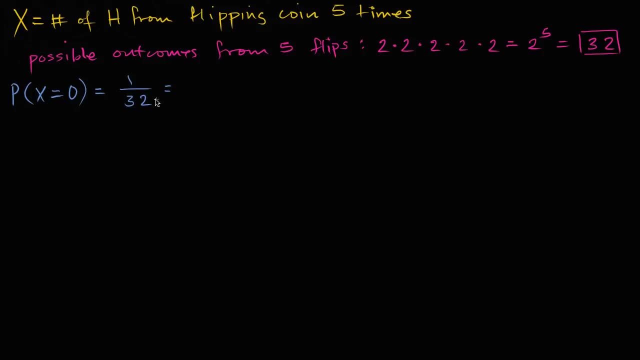 for the binomial distribution. so you get a sense of where the name comes from. Let's write it in those terms: So this one, this one, this one right over here, the way, one way to think about that in combinatorics. 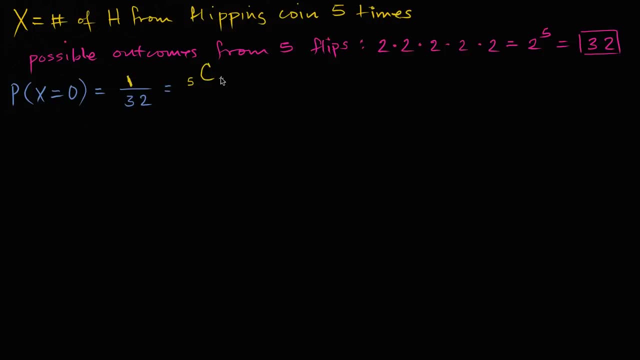 is that you had five flips and you're choosing zero of them to be heads. Five flips and you're choosing zero of them to be heads. And let's verify that five choose zero is indeed one. So five choose zero. let me write it right over here. 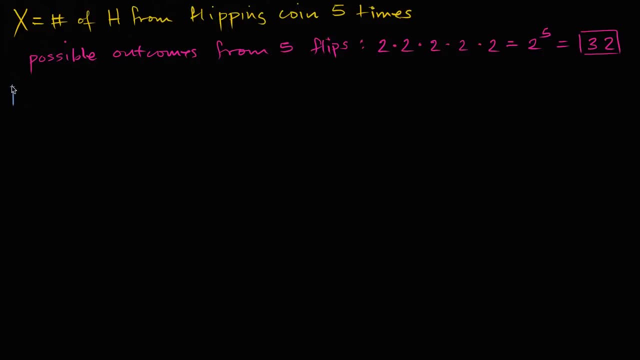 Let me do it in. I'll start with this, I'll start in blue, all right. So let's think about the probability that our random variable x is equal to one. Well, actually, let me start with zero. The probability that our random variable x. 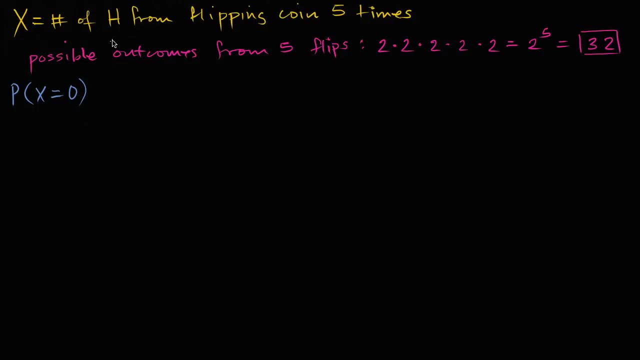 is equal to zero. So that would mean that you got no heads out of the five flips. Well, there's only one way- one out of the 32 equally likely possibilities- that you get no heads, That's the one where you just get five. 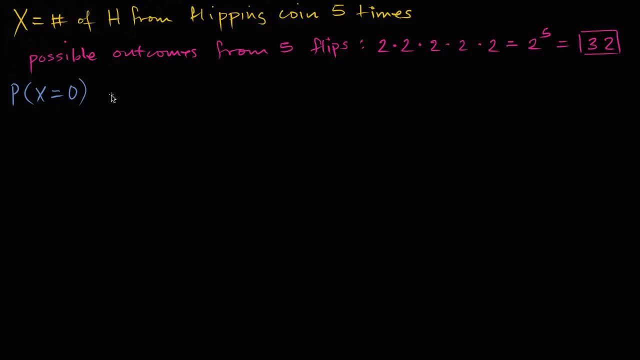 where you get five tails. So this is just going to be, this is going to be equal to one out of the 32 equally likely possibilities. Now for this case, you know to kind of think in terms of kind of the binomial coefficients. 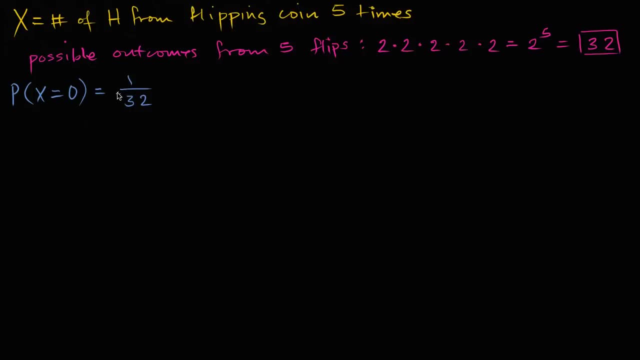 and combinatorics and all of that. it's much easier to just reason through it. But just so we can think in those terms and it'll be more useful as we go into higher values for our random variable. And it's also. this is all a buildup. 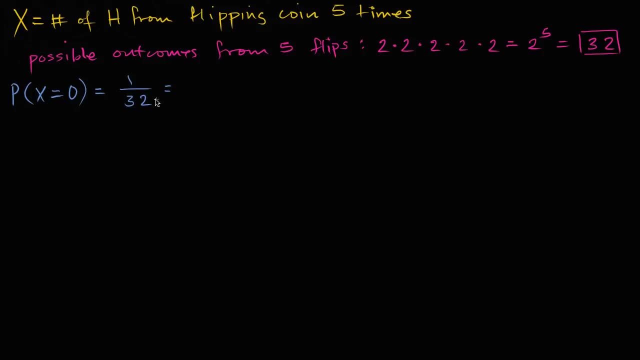 for the binomial distribution. so you get a sense of where the name comes from. Let's write it in those terms: So this one, this one, this one right over here, the way, one way to think about that in combinatorics. 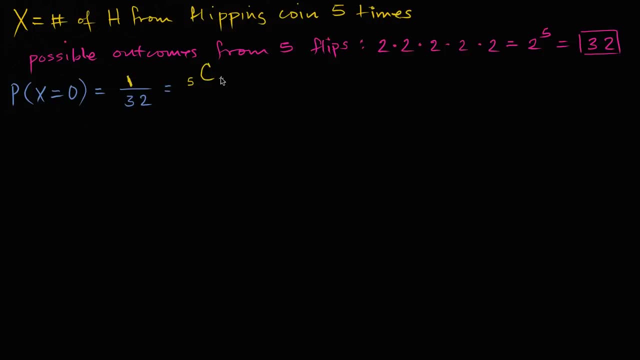 is that you had five flips and you're choosing zero of them to be heads. Five flips and you're choosing zero of them to be heads. And let's verify that five choose zero is indeed one. So five choose zero. let me write it right over here. 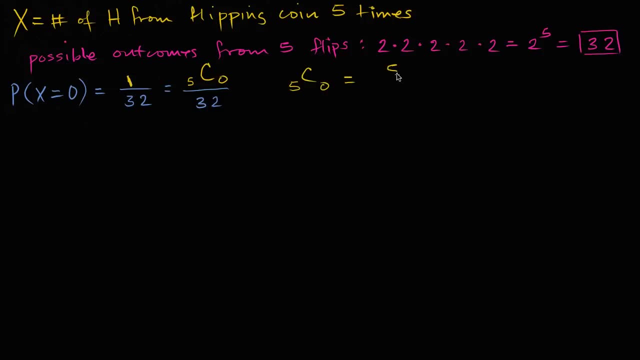 Five, choose zero. Zero is equal to five factorial over over over. five minus zero factorial over actually over zero factorial times. five minus zero factorial. Five minus zero factorial. Well, this is zero. factorial is one by definition, and so this is going to be five factorial. 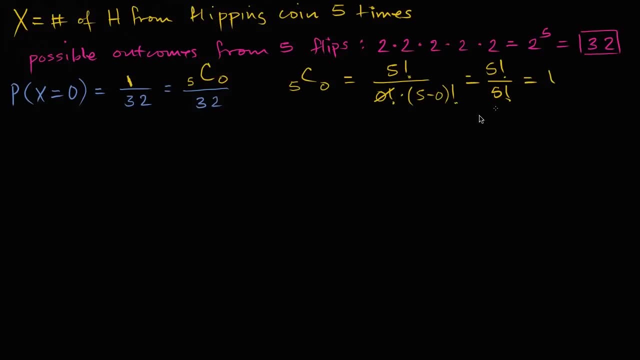 over five factorial, which is going to be equal to one. Once again, I like reasoning through this. I like reasoning through it instead of blindly applying a formula. but I just wanted to show you that these two ideas are consistent. So let's keep going and I'm gonna do. x equals one. 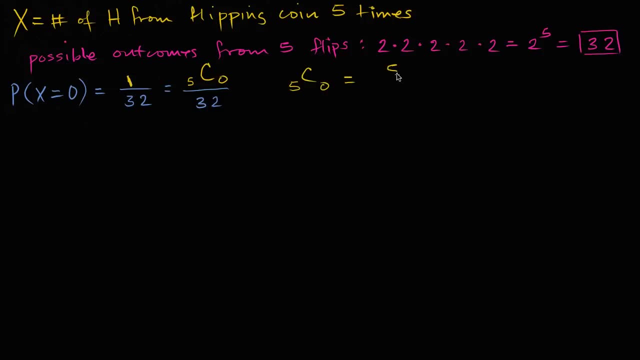 Five, choose zero. Zero is equal to five factorial over over over. five minus zero factorial over actually over zero factorial times. five minus zero factorial. Five minus zero factorial. Well, this is zero. factorial is one by definition, and so this is going to be five factorial. 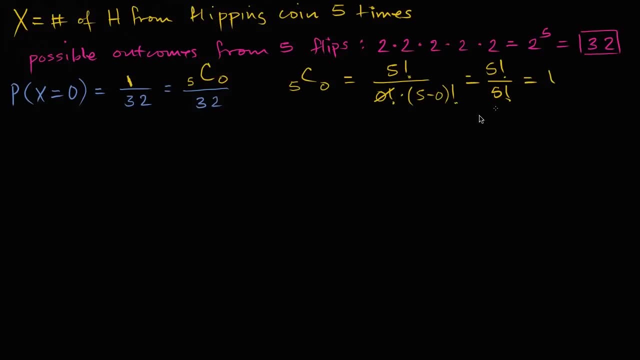 over five factorial, which is going to be equal to one. Once again, I like reasoning through this. I like reasoning through it instead of blindly applying a formula. but I just wanted to show you that these two ideas are consistent. So let's keep going and I'm gonna do. x equals one. 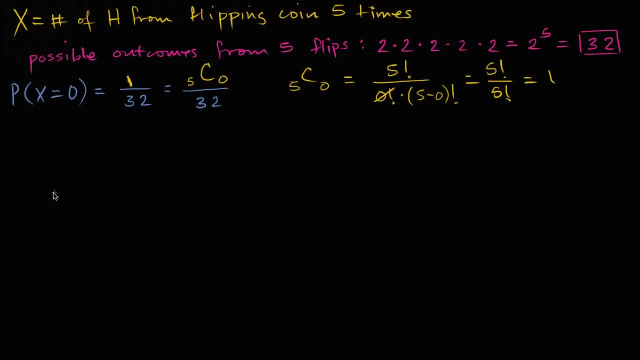 all the way up to x equals five. and if you are inspired- and I encourage you to be inspired- I try to fill out the whole thing. What's the probability that x equals one, two, three, four or five? So let's go to the probability that x equals two. 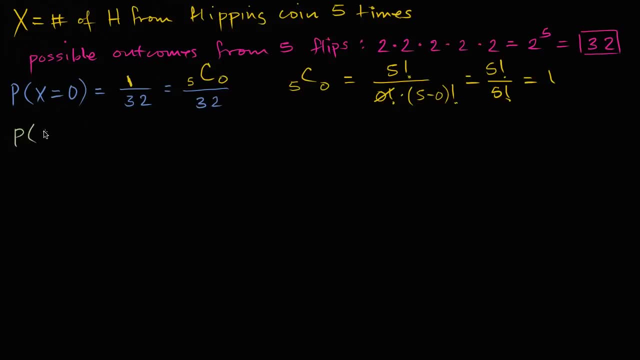 oh sorry, x equals one, So the probability that x equals one is going to be equal to. well, how do you get one head? Well, it could be the first, one could be head, and then the rest of them are gonna be tails. 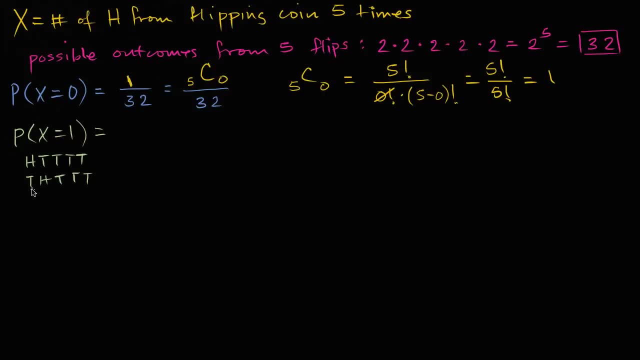 The second one could be head, and then the rest of them are going to be tails. I could write them all out, but you could see that there's just five different places for it to have that one head. So five out of the 32 equally likely outcomes. 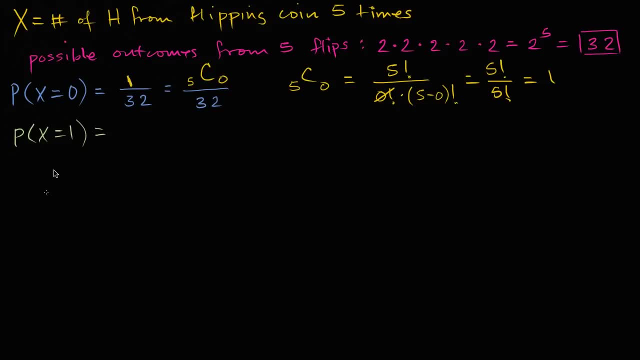 involve one head, So let me write that down. So this is going to be equal to: this is going to be equal to five out of the 32 equally likely outcomes, which, of course, is the same thing. this is going to be the same thing as saying: 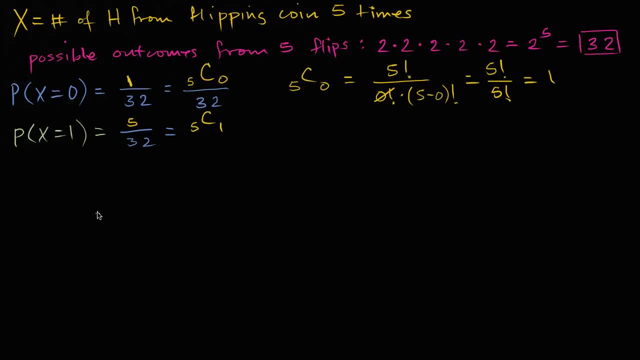 look, I got five flips and I'm choosing one of them. I'm choosing one of them to be heads, So that over 32, and you could verify that- five factorial over one factorial times five minus actually. let me just do it. 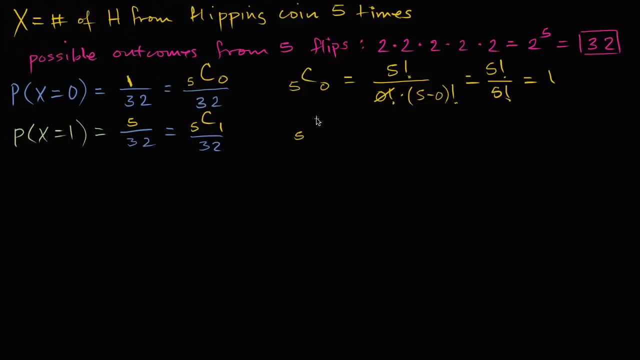 just so that you don't have to take my word for it. So five- choose one- is equal to five factorial over one factorial, which is just one times five minus four, sorry, five minus one factorial, which is equal to five factorial over four factorial. 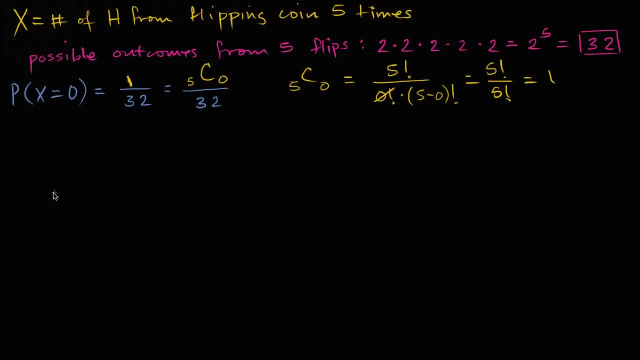 all the way up to x equals five. and if you are inspired- and I encourage you to be inspired- I try to fill out the whole thing. What's the probability that x equals one, two, three, four or five? So let's go to the probability that x equals two. 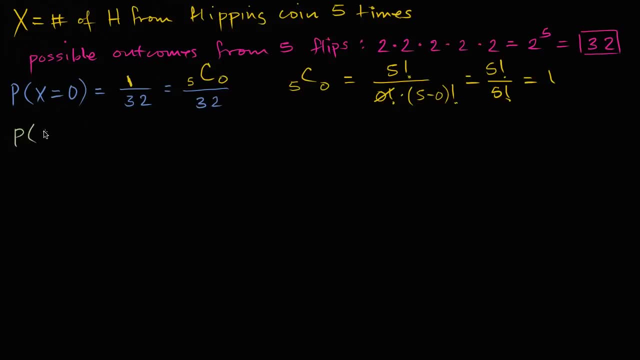 oh sorry, x equals one, So the probability that x equals one is going to be equal to. well, how do you get one head? Well, it could be the first, one could be head, and then the rest of them are gonna be tails. 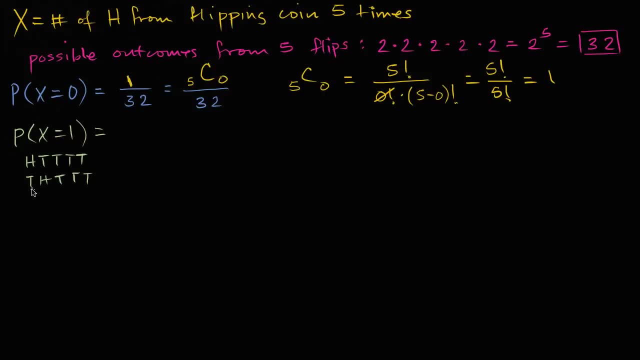 The second one could be head, and then the rest of them are going to be tails. I could write them all out, but you could see that there's just five different places for it to have that one head. So five out of the 32 equally likely outcomes. 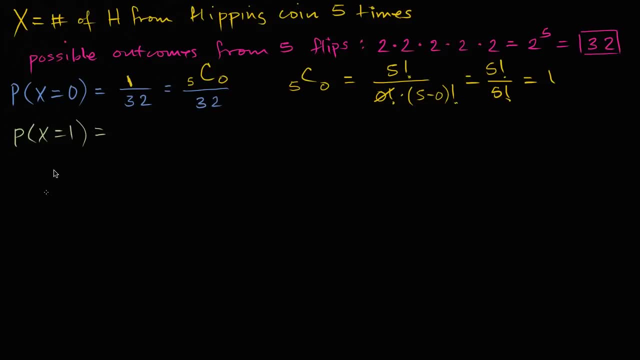 involve one head, So let me write that down. So this is going to be equal to: this is going to be equal to five out of the 32 equally likely outcomes, which, of course, is the same thing. This is going to be the same thing as saying: 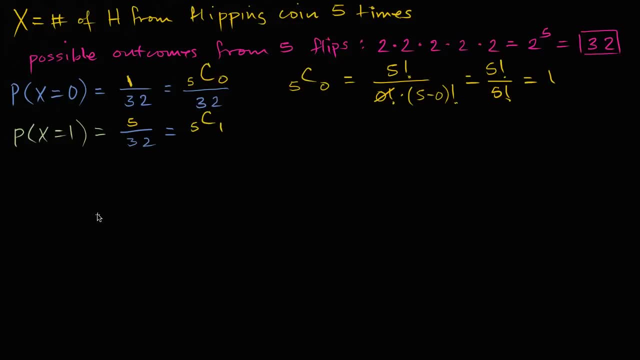 look, I got five flips and I'm choosing one of them. I'm choosing one of them to be heads, So that over 32.. And you could verify that: five factorial over one factorial times five minus actually. let me just do it. 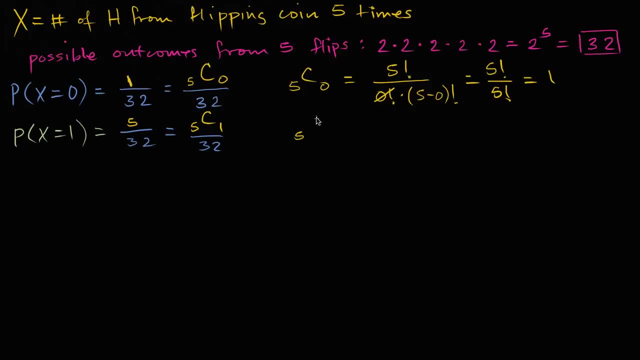 just so that you don't have to take my word for it. So five- choose one- is equal to five factorial over one factorial, Which is just one Times five minus four, sorry, five minus one factorial, Which is equal to five factorial over four factorial. 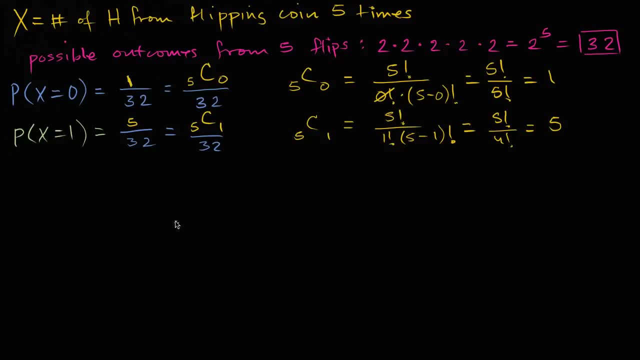 Which is just going to be equal to five. All right, we're making good progress, So now let in purple. let's think about the probability that our random variable x is equal to two. Well, this is going to be equal to. 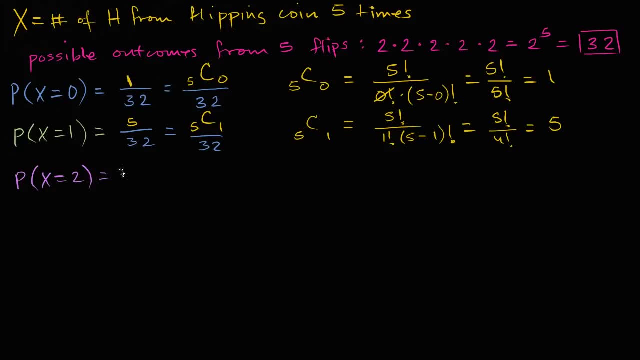 and now I'll actually resort to the combinatorics. So this is: you have five flips and you're choosing two of them to be heads over 32 equally likely possibilities. So this is the number of possibilities that result in two heads. 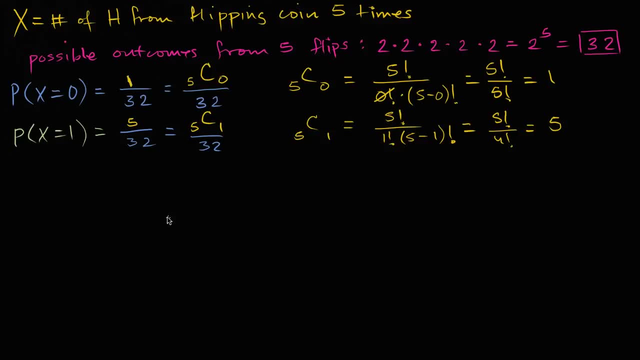 which is just going to be equal to five. All right, we're making good progress, So now let in purple. let's think about the probability that our random variable x is equal to two. Well, this is going to be equal to. 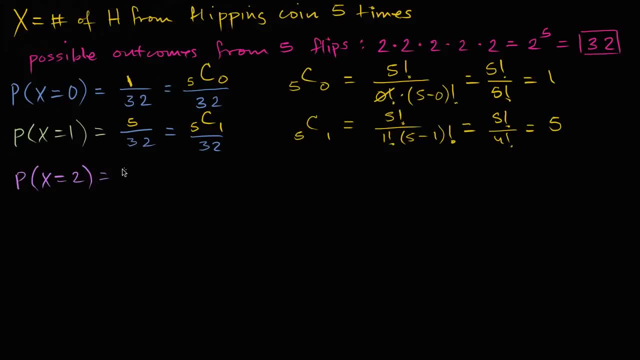 and now I'll actually resort to the combinatorics. so this is: you have five flips and you're choosing two of them to be heads over 32 equally likely possibilities. So this is the number of possibilities that result in two heads. 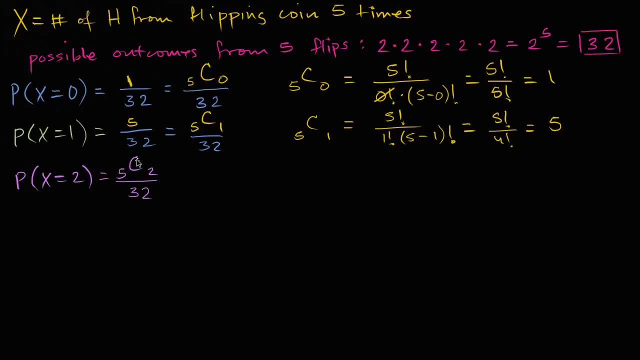 Two of the five flips have chosen to be heads. I guess you could think of it that way- by the random gods or whatever you want to say, And that's so. this is the fraction of the 32 equally likely possibilities. so this is the probability that x equals two. 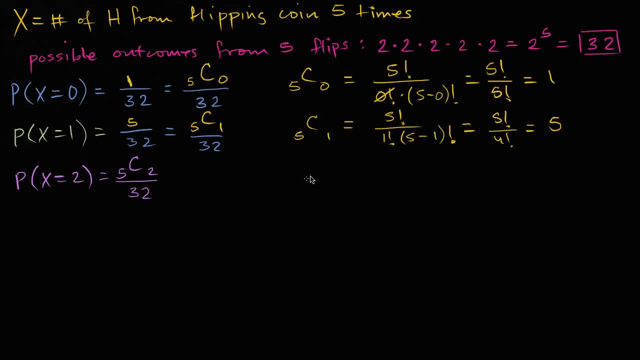 Well, what's this going to be? Well, I'll do it right over here, and actually no reason for me to have to keep switching colors. So five choose two is going to be equal to five factorial over two factorial times five minus two factorial. 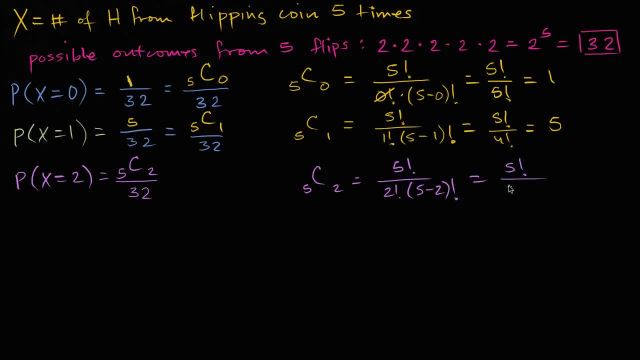 Five minus two factorial. so this is five factorial over two factorial, times three factorial. And this is going to be equal to five times four times three, times two. I could write times one, but that doesn't really do anything for us- And then two factorial is just going to be two. 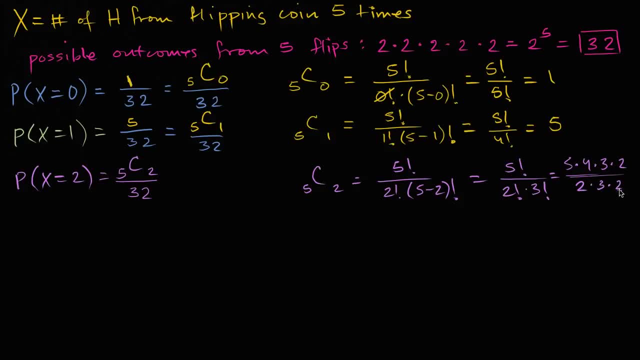 and then the three. factorial is three times two. I could write times one, but once again doesn't do anything for us. That cancels with that. Four divided by two is two. Five times two is 10.. So this is equal to 10.. 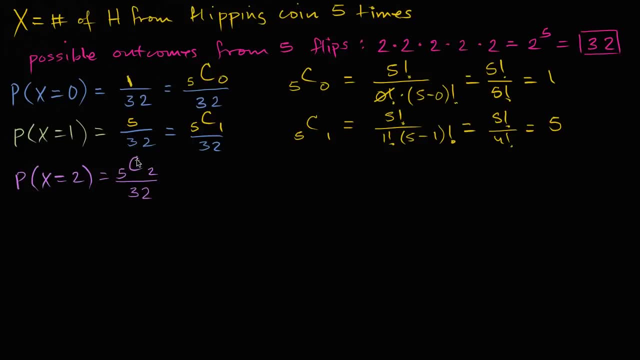 Two of the five flips have chosen to be heads. I guess you could think of it that way- by the random gods or whatever you want to say. And that's so. this is the fraction of the 32 equally likely possibilities. So this is the probability that x equals two. 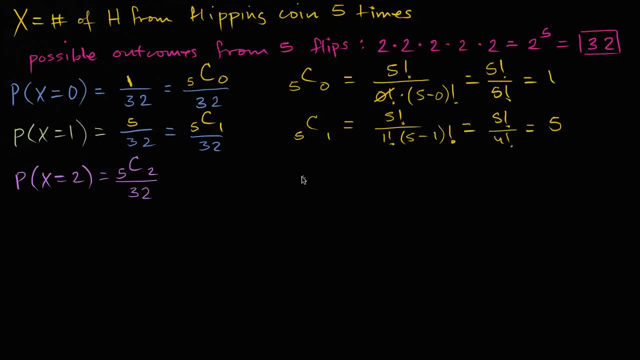 Well, what's this going to be? Well, I'll do it right over here, And actually no reason for me to have to keep switching colors. So five choose two is going to be equal to five factorial over two factorial times five minus two factorial. 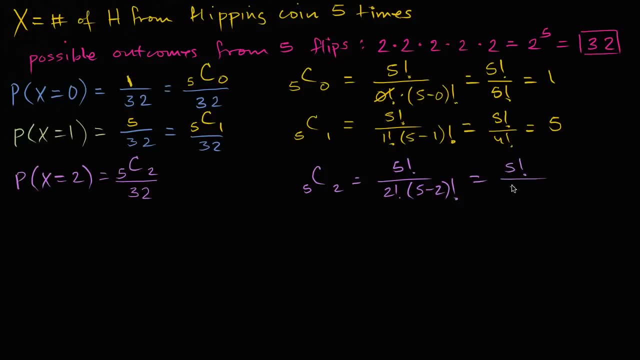 Five minus two factorial. So this is five factorial over two factorial, times three factorial. And this is going to be equal to five times four times three, times two. I could write times one, but that doesn't really do anything for us- And then two factorial is just going to be two. 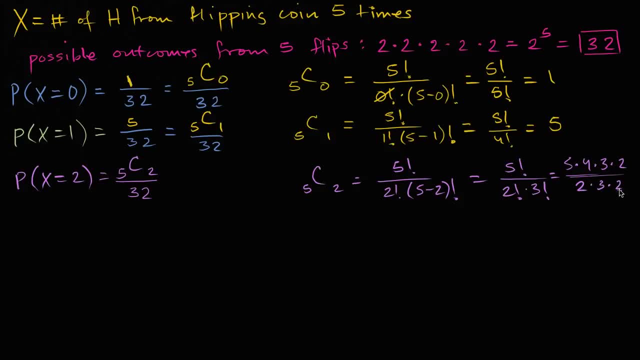 And then the three factorial is three times two. I could write times one, but once again doesn't do anything for us. That cancels with that. Four divided by two is two. Five times two is 10.. So this is equal to 10.. 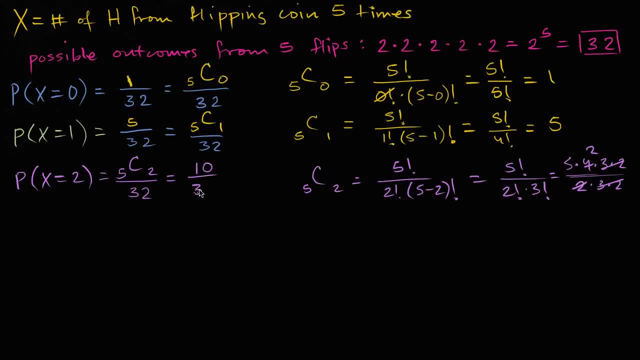 This right over here is equal to 10- 30 seconds, 10- 30 seconds, And obviously we could simplify this fraction, but I like to leave it this way, because we're now thinking everything is in terms of 30 seconds. There's a one 30 second chance. 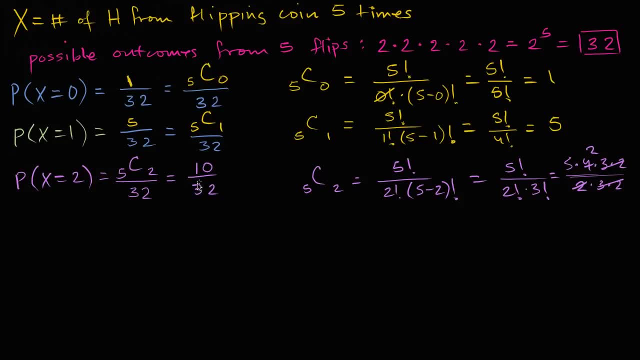 x equals zero, Five 30 seconds chance that x equals one And a 10 30 seconds chance that x equals two. Let's keep on going. All right, I'll go in orange. So what is the probability that our random variable x is equal to three? 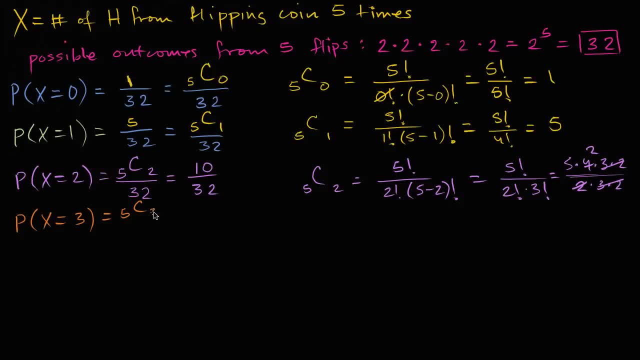 Well, this is going to be five Out of the five flips. we're going to need to choose three of them to be heads, to figure out which of the possibilities involve exactly three heads. And this is over two equally likely possibilities, And this is going to be equal to: 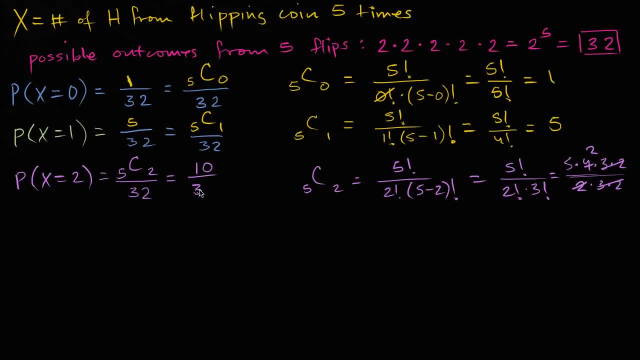 This right over here is equal to 10- 30 seconds, 10- 30 seconds, And obviously we could simplify this fraction, but I like to leave it this way, because we're now thinking everything is in terms of 30 seconds. 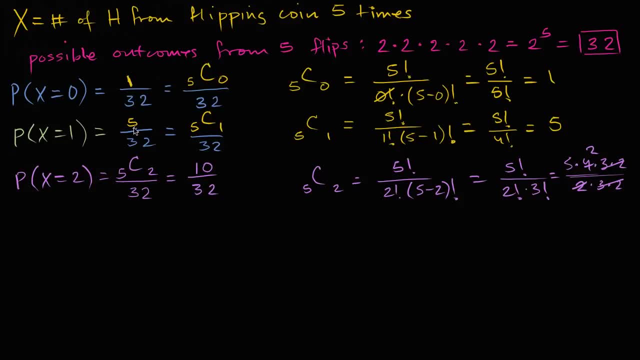 There's a one 30 second chance- x equals zero, Five 30 seconds chance that x equals one and a 10 30 seconds chance that x equals two. Let's keep on going. All right, I'll go in orange. 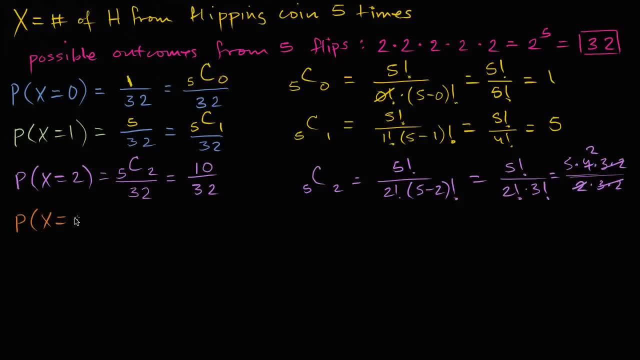 So what is the probability that our random variable x is equal to three? Well, this is going to be five. out of the five flips, we're gonna need to choose three of them to be heads, to figure out which of the possibilities involve exactly three heads. 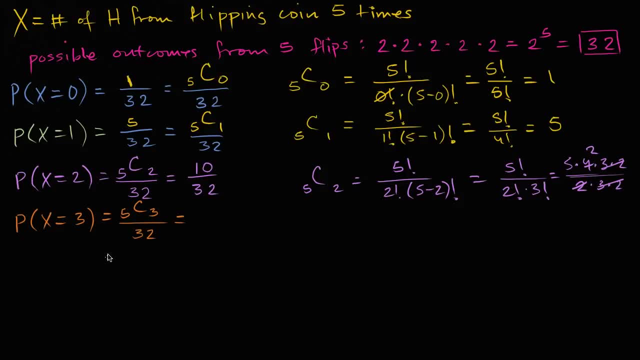 And this is over two equally likely possibilities, And this is going to be equal to: so five- choose three is equal to five factorial over three factorial times five minus three factorial. Actually, let me just write it down: Five minus three factorial, which is equal to five factorial. 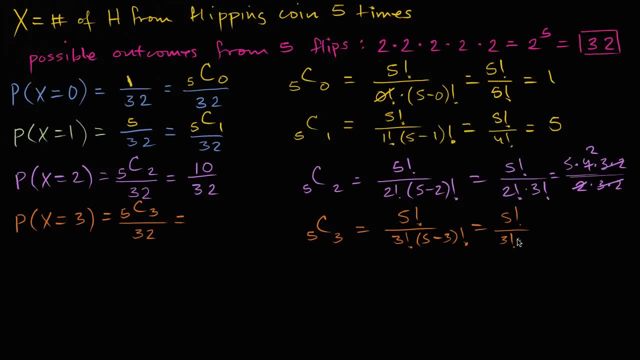 over three factorial times. two factorial Times, two factorial. Well, that's exactly what we had up here. We just swapped the three and the two. So this also is going to be equal to 10.. So this is also going to be equal to 10- 30 seconds. 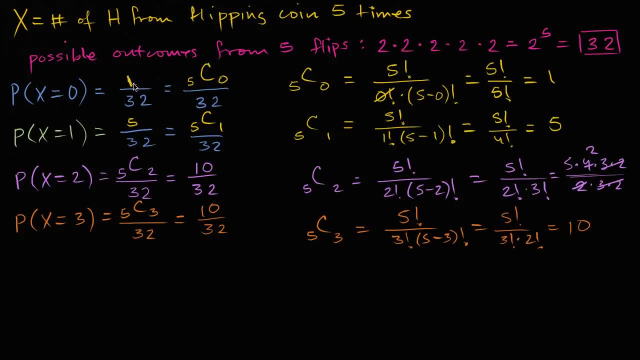 All right, two more to go And I think you're gonna start seeing a little bit of a symmetry here. One, five, 10, 10.. Let's keep going, Let's keep going, and I haven't used white yet. 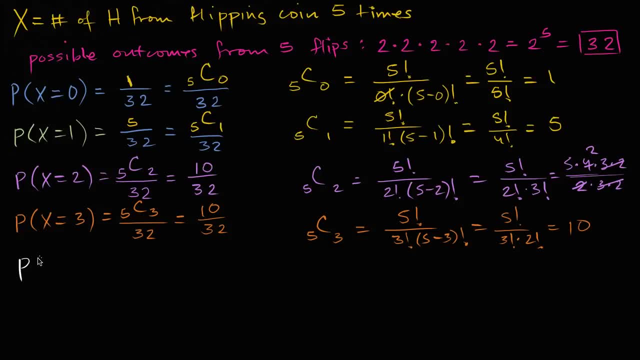 so maybe I'll use white The probability, the probability that our random variable x is equal to four. Well, out of our five flips, we wanna select four of them to be heads. or out of the five, yeah, four, and we wanna see. 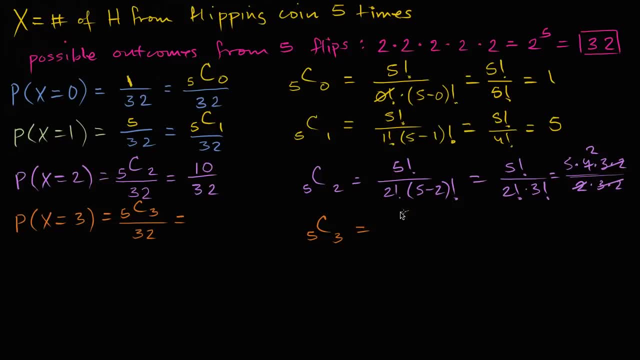 so five choose three is equal to five factorial over three factorial times five minus three factorial. Actually, let me just write it down: Five minus three factorial, which is equal to five factorial over three factorial times two factorial Times two factorial. Well, that's exactly what we had up here. 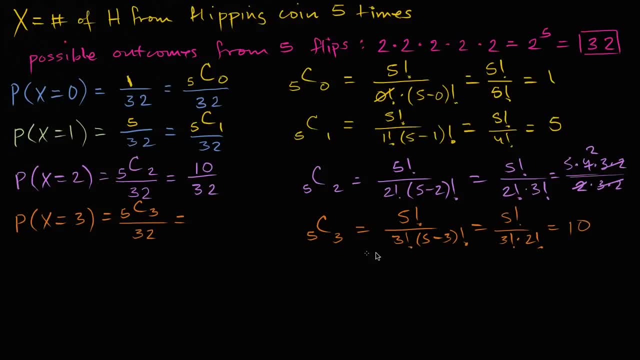 We just swapped the three and the two, So this also is going to be equal to 10.. So this is also going to be equal to 10, 30 seconds. All right, two more to go And I think you're going to start seeing. 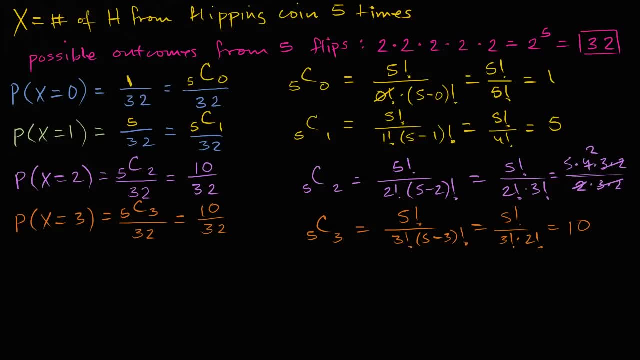 a little bit of a symmetry here: One, five, 10,, 10.. Let's keep going, Let's keep going. And I haven't used white yet, so maybe I'll use white: The probability, the probability that our random variable x. 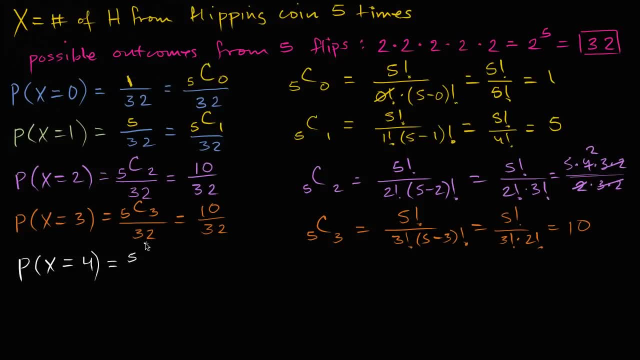 is equal to four. Well, out of our five flips, we want to select four of them to be heads. So we're out of the five, yeah, four, and we want to see. let me you know we're obviously not actively selecting. 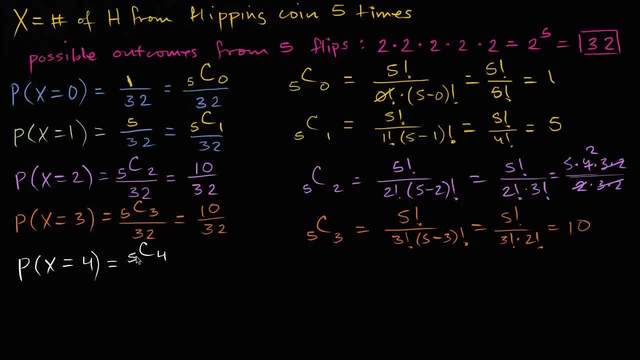 One way to think about it. we want to figure out the possibilities that involve: out of the five flips, four of them are chosen to be heads, or four of them are heads, And this is over 32 equally likely possibilities. So five, choose four. 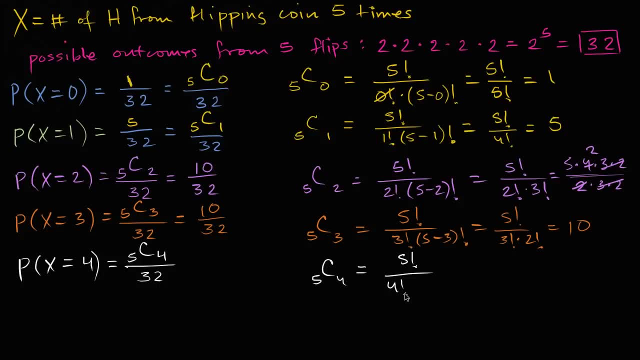 is equal to five factorial over four factorial times five minus four factorial, which is equal to well, that's just going to be five factorial. This is going to be one factorial right over here, So that doesn't change the value of the. 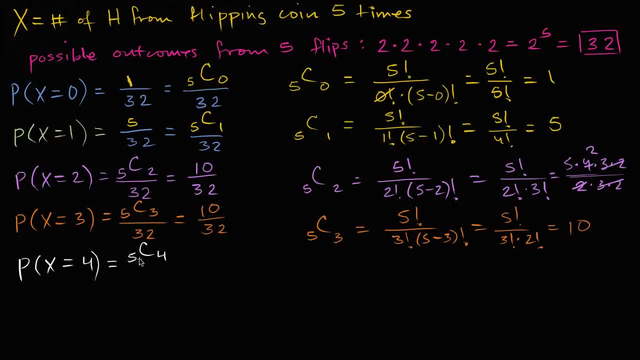 let me you know we're obviously not actively selecting One way to think about it. we wanna figure out the possibilities that involve, out of the five flips, four of them are chosen to be heads, or four of them are heads, And this is over 32 equally likely possibilities. 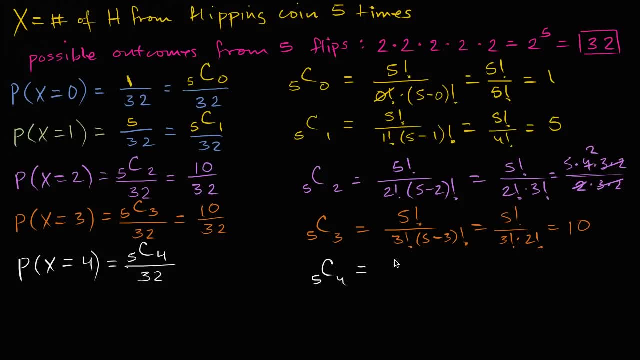 So five, choose four, is equal to five factorial over four factorial times five minus four factorial, which is equal to well, that's just gonna be five factorial. This is gonna be one factorial right over here, So that doesn't change the value of the. 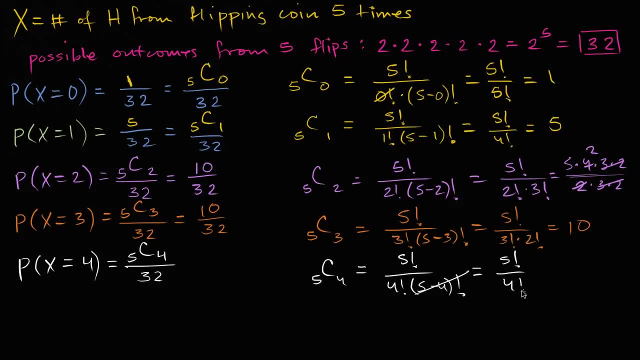 you're just gonna multiply one factorial times four factorial, so it's five factorial over four factorial, which is equal to five. So once again this is 532nds And you could have reasoned through this, because if you're saying you want five heads, 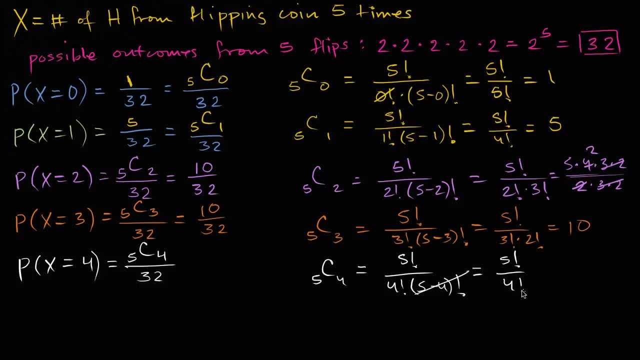 you're just going to multiply one factorial times four factorial, So it's five factorial over four factorial, which is equal to five. So once again, this is 5, 30 seconds And you could have reasoned through this, because if you're saying you want five heads, 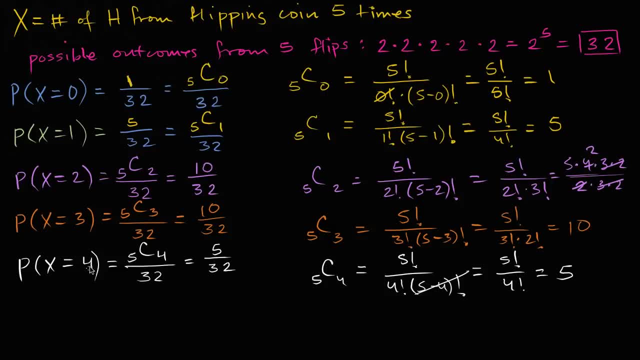 that means you have one tail And that, and there's only five. there's five different places. you could put that: one tail, Five, there are five possibilities with one tail, Five of the 32 equally likely. And then, and you could probably guess, 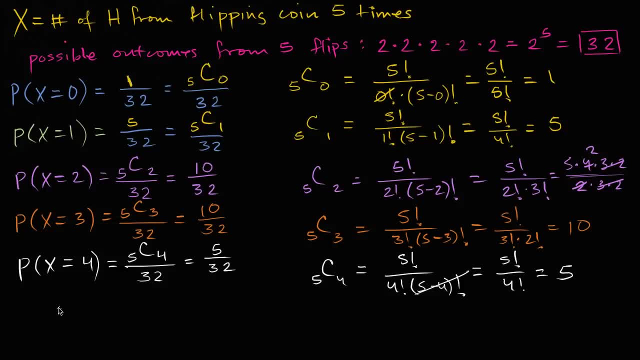 what we're going to get for x equals five, Because having five heads means you have zero tails and there's only going to be one possibility out of the 32 with zero tails or that have all heads. Let's write that down. 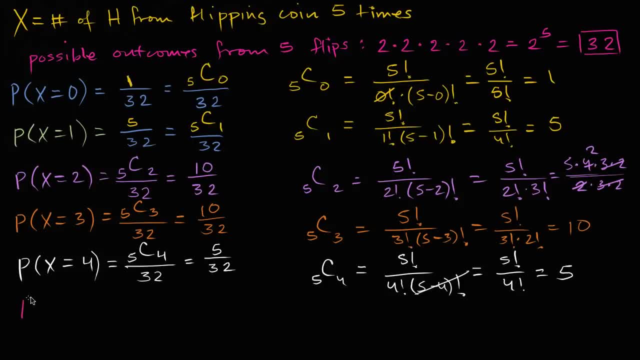 So the probability, the probability that a random variable x is equal to five. So we have all five heads And you could say this is five and we're choosing five of them to be heads. Okay, Out of the 32 equally likely possibilities. 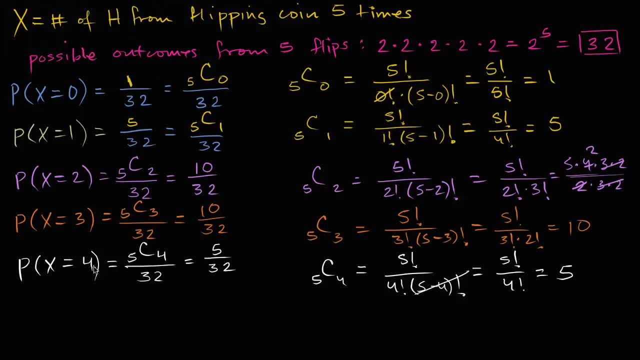 that means you have one tail And there's only five. there's five different places you could put that: one tail Five. there are five possibilities with one tail, five of the 32 equally likely. And then, and you could probably guess, 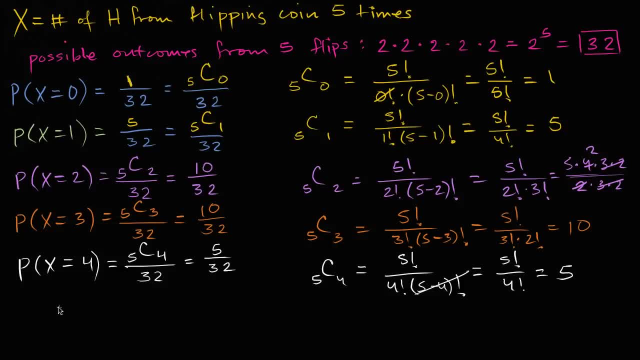 what we're gonna get for x equals five, because having five heads means you have zero tails and there's only going to be one possibility out of the 32 with zero tails or that have all heads. Let's write that down. So the probability. 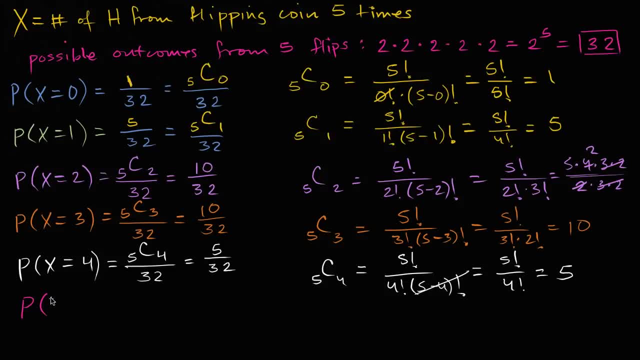 the probability that a random variable x is equal to five. so we have all five heads And you could say: this is five and we're choosing five of them to be heads, and we're choosing five of them to be heads and we're choosing five of them to be heads. 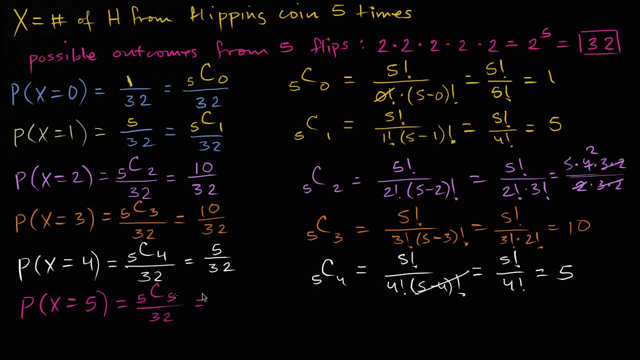 out of the 32 equally likely possibilities. Well, five choose five. that's going to be actually- let me just write it here, since I've done it for all of the other ones: Five choose five is five factorial over five factorial. 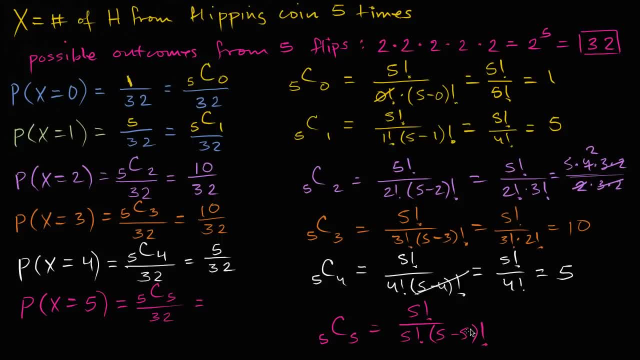 times five minus five factorial. Well, this right over here is zero factorial, which is equal to one, and so this whole thing simplifies to one. So this is going to be one out of one thirty seconds, And so you see the symmetry. 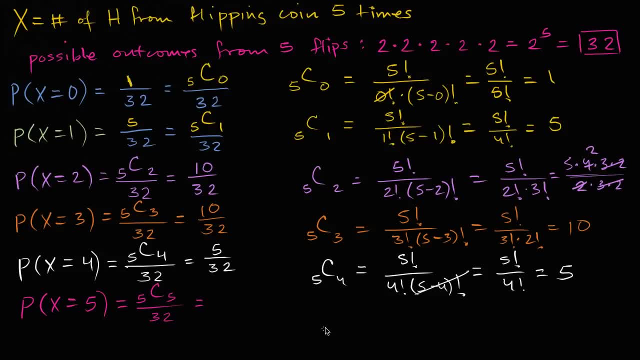 Well, five choose five that's going to be actually. let me just write it here, since I've done it for all of the other ones: Five choose five is five factorial over five factorial times five minus five factorial. Well, this right over here is zero factorial. 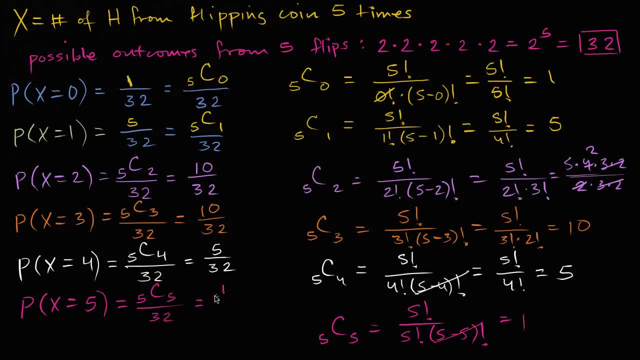 which is equal to one, And so this whole thing simplifies to one. So this is going to be one out of one 30 seconds, And so you see the symmetry: one 30 second, one 30 seconds, Five 30 seconds. 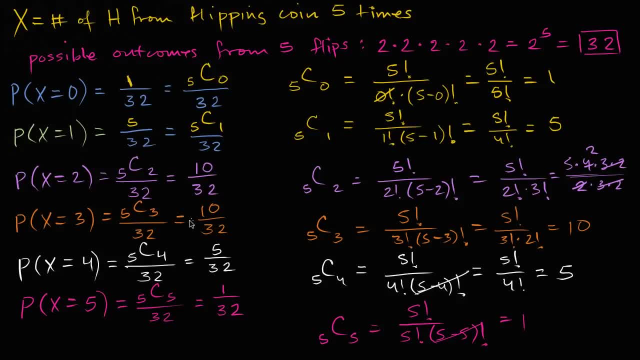 five 30 seconds, 10, 30 seconds, 10, 30 seconds. And that makes sense because the probability of getting five heads is the same as the probability of getting zero tails, And the probability of getting zero tails should be the same as the probability. 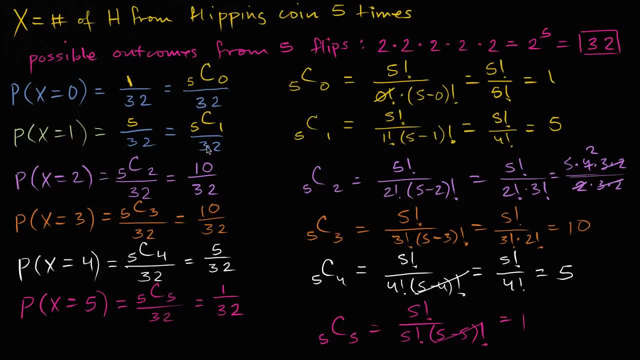 of getting zero heads. So I'll leave you there for this video. In the next video we'll kind of graphically represent this and we'll see the probability distribution for this random variable. 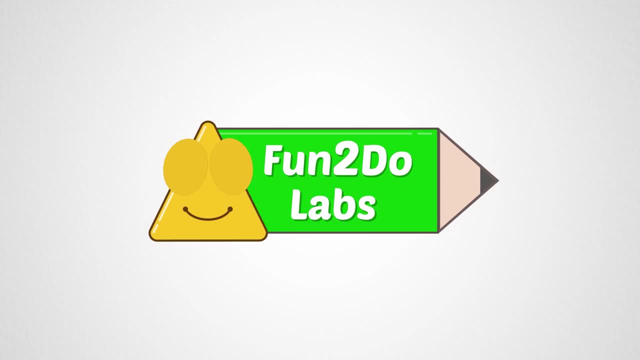 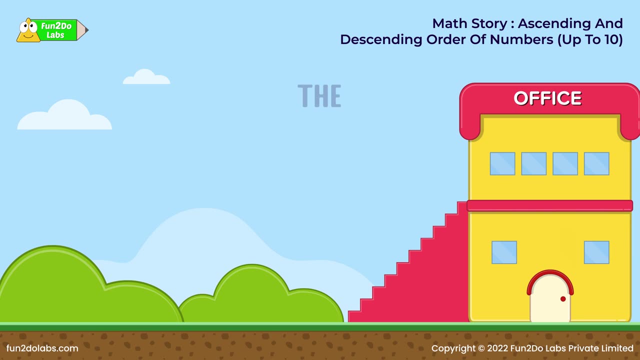 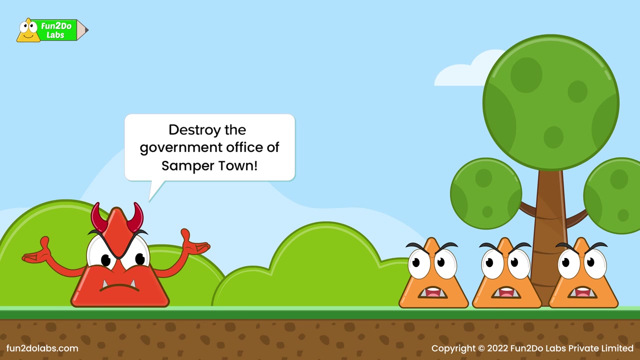 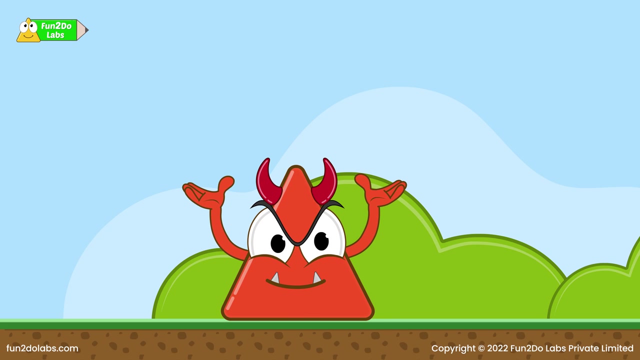 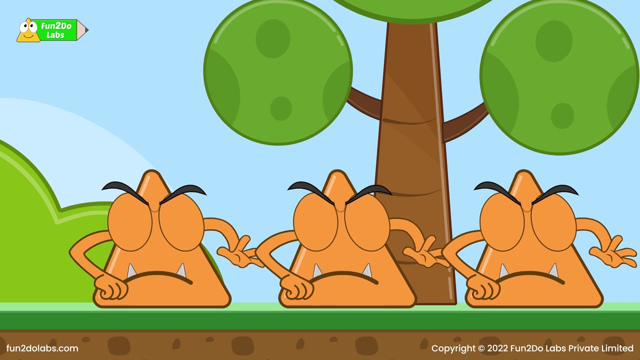 Math Story Ascending and descending order of numbers up to 10. The Office Attack: Destroy the government office of Sampatown. We need to show our power to them. I am Atriha Boss, the smartest villain you will ever come across. Yes, boss, Long live Atriha Boss. 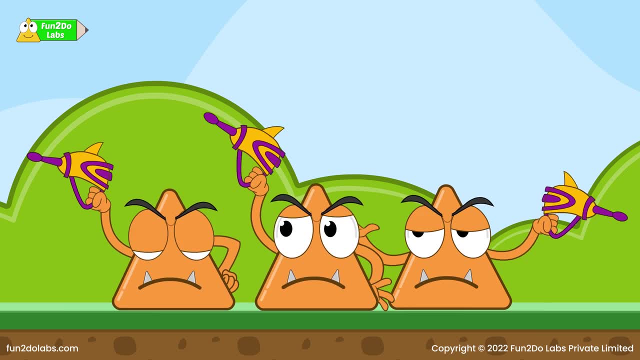 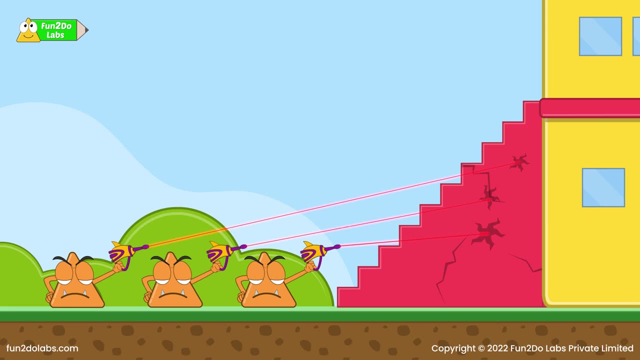 Says the Atriha gang, They are ready to follow their boss's order. Soon Atriha gang reaches the town, They start attacking the government office building. Dryo and Squero, who were passing by, are shocked to see this. 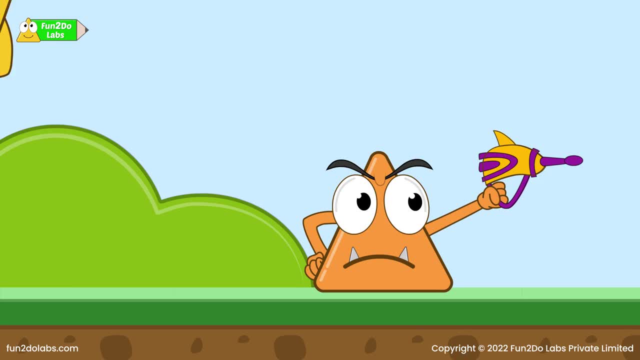 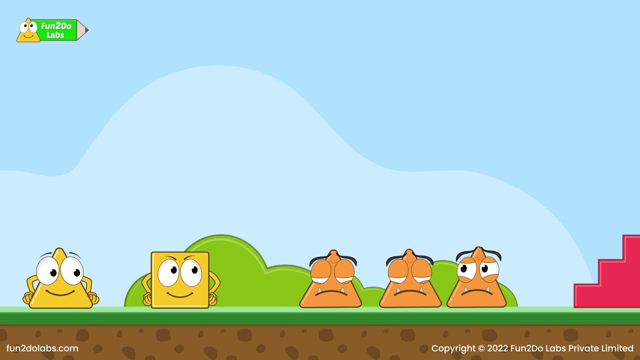 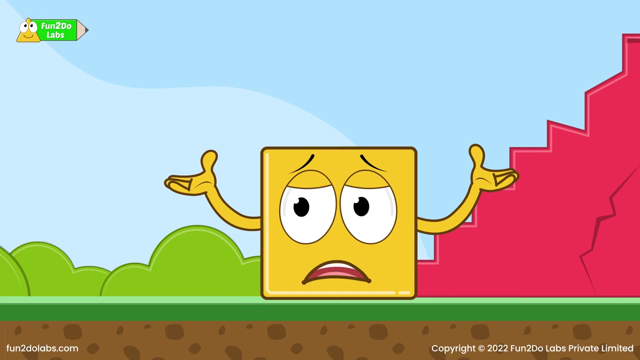 We need to stop them. Bang Boom, Crash Boom. Both of them fight Atriha gang bravely. The bad robots run away to save themselves. Look at the steps, Atriha, They damaged them completely. The government officers will find it difficult to reach the second floor now.